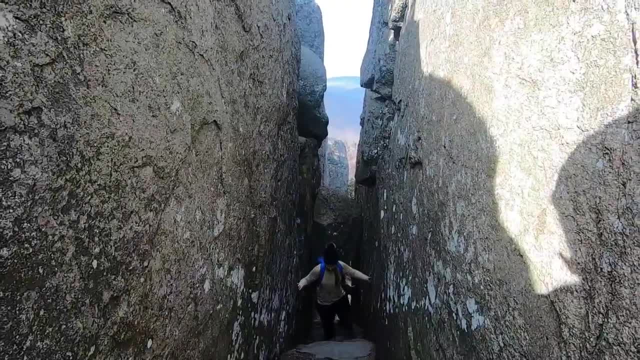 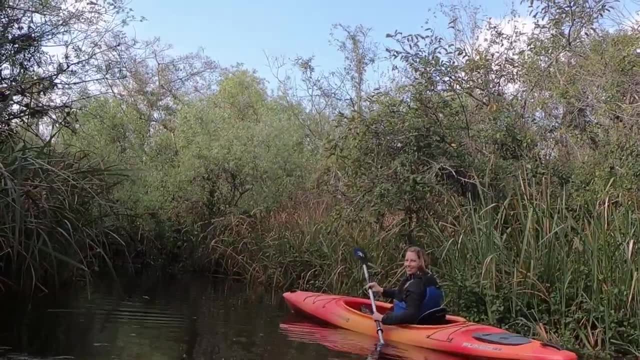 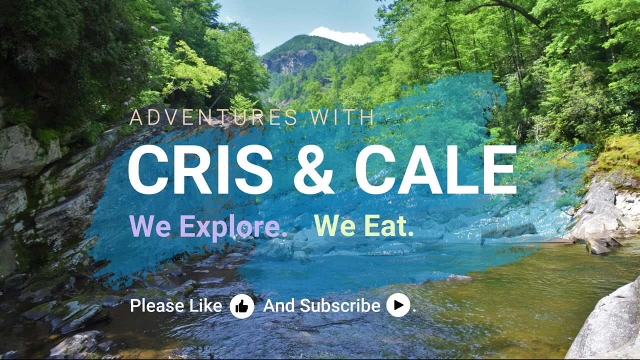 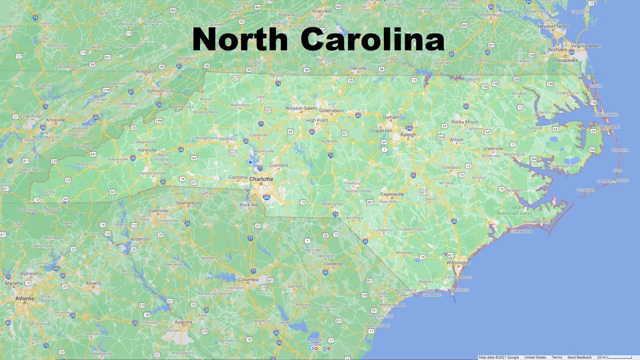 We crushed the gnarly hike Wow. In July, my daughter Joelle and I hiked the tallest peak east of the Mississippi. We summited Mount Mitchell, a peak in western North Carolina contained within one of the nation's first state parks. 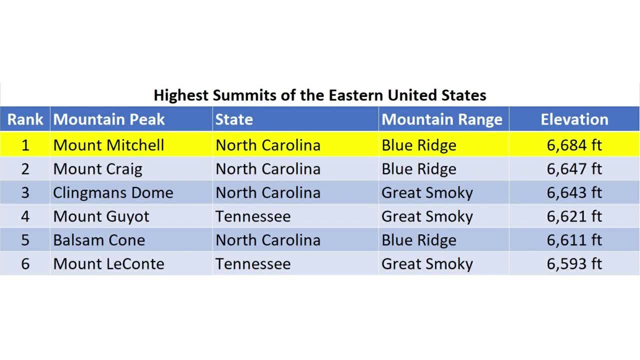 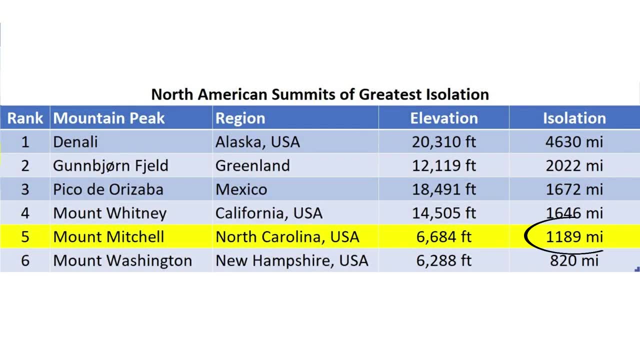 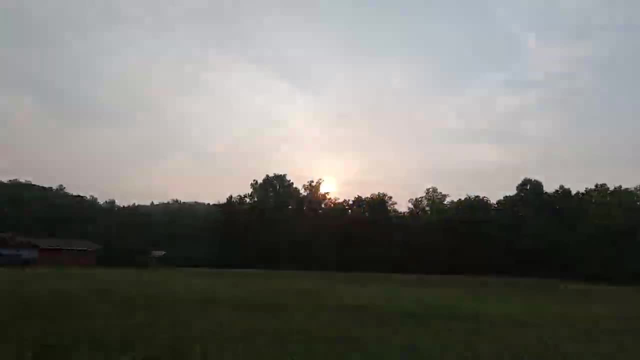 Not only is Mount Mitchell the highest of all summits in the eastern United States, it is the fifth most isolated peak in all of North America, almost 1,200 miles from another peak of its size. It stands at 6,684 feet and provides great views of the surrounding Blue Ridge Mountains. 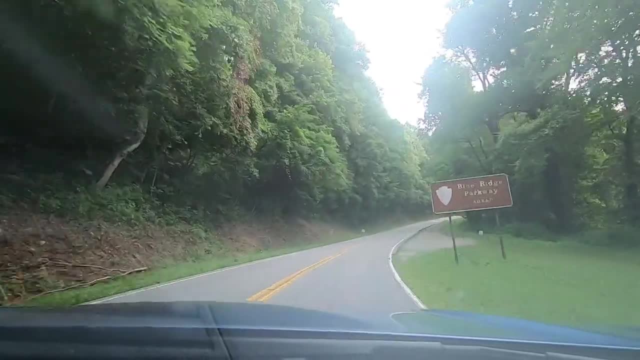 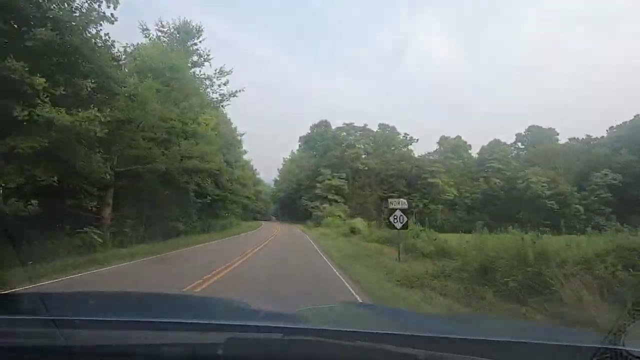 Due to the high elevation and prominence, weather at the top can be severe. Average annual snowfall is 75 inches and winds up to 178 miles per hour have been recorded there. Our day, however, brought beautiful, modest summer weather. 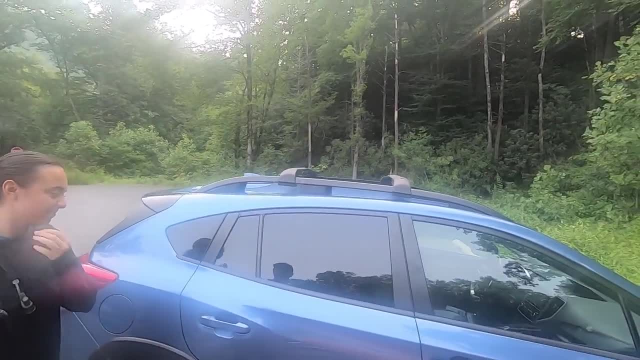 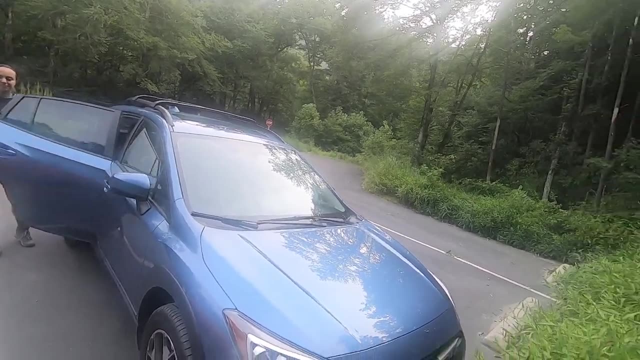 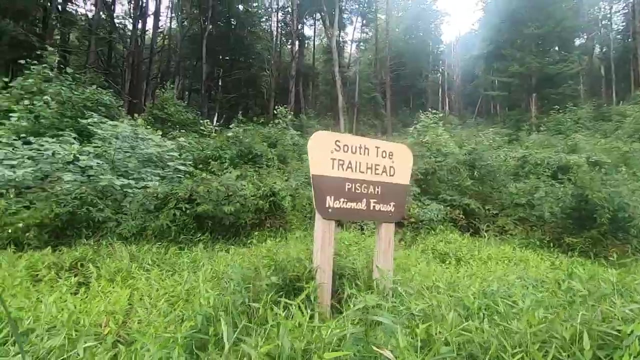 So here we are. We have a guest Subaru today. This is Dory. This is Dory. This is Joella's Subaru. Very nice. So this is where we parked at the South Tove Trailhead. That's it There. 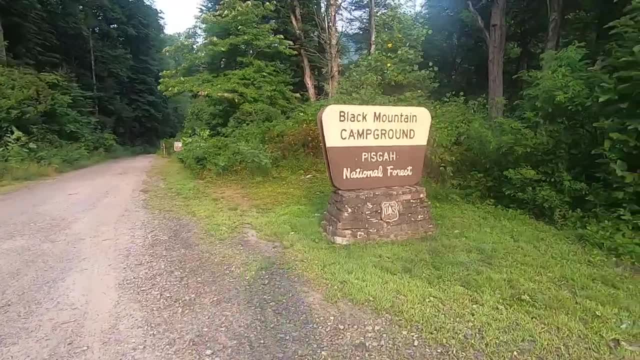 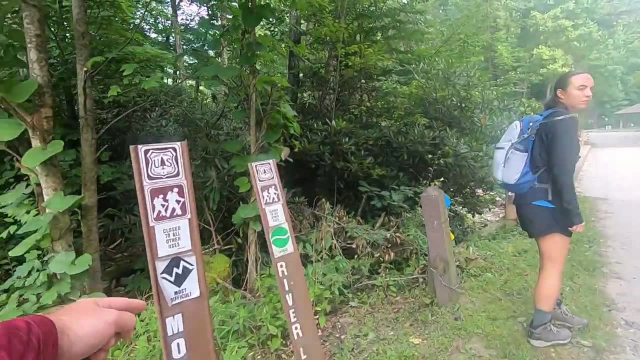 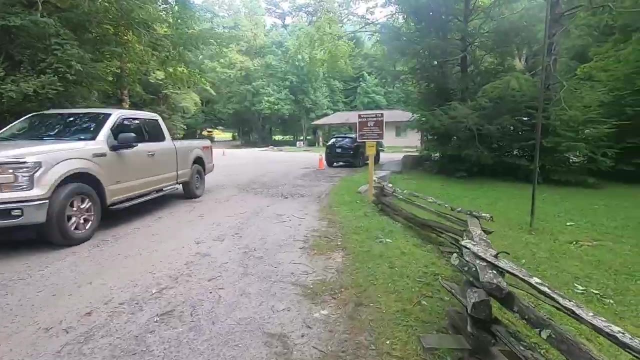 See, Mount Mitchell, We're here. We've got six miles. This is the Mount Mitchell Trail right here, Most difficult. What does that mean? I guess that it means it's difficult. Welcome to bear country. Yeah, There it is. 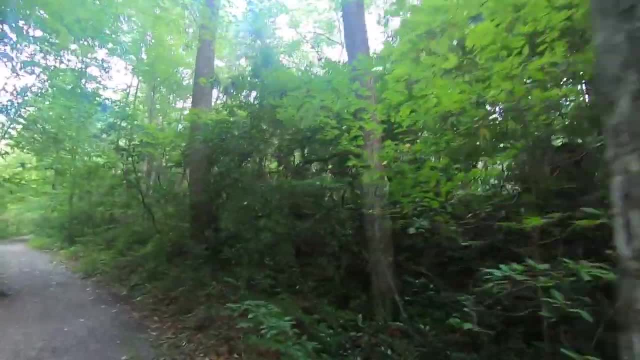 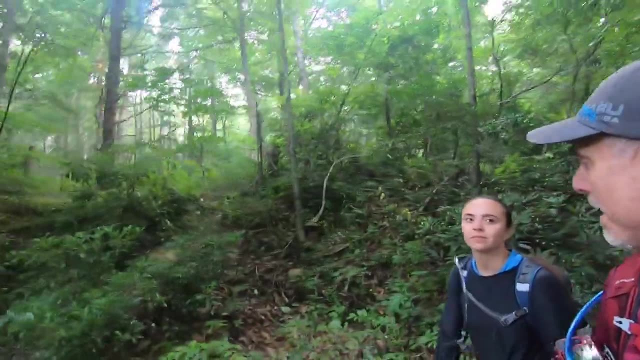 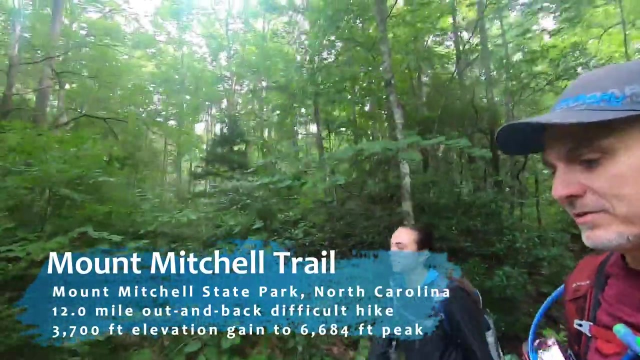 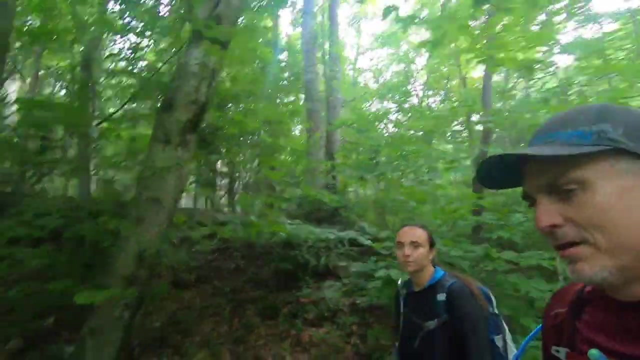 Okay, Well, Mitchell, Yeah, There We're taking the blue. We are starting out right here at the Black Mountain Campground And we are beginning our trek up 3,600 feet. It's about just under six miles to Mount Mitchell. 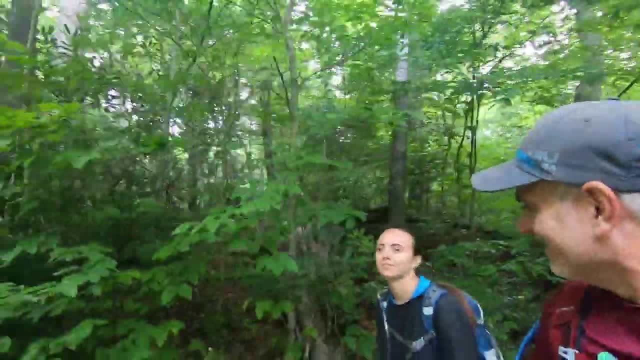 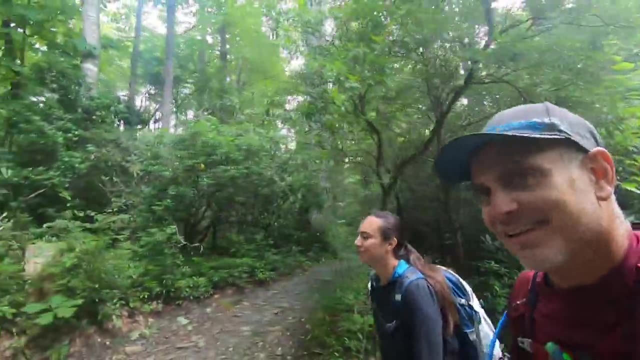 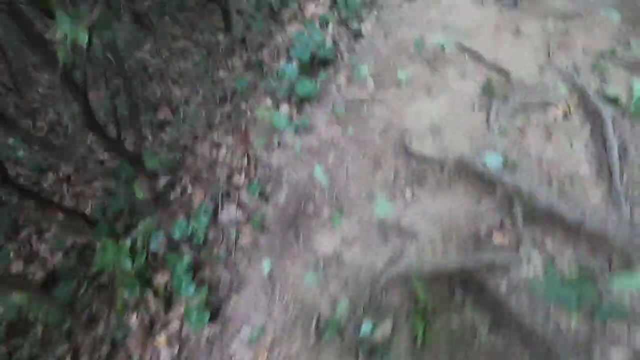 How do you feel about this trek? I'm a little nervous, But it feels really good. I think we'll be fine. You said about 60, 65 degrees. Yeah, So a half mile and 200 foot elevation, Okay. 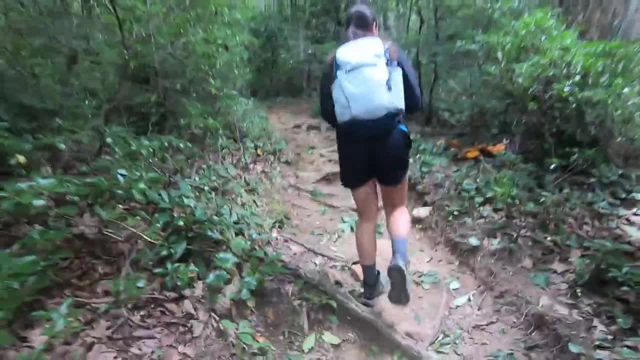 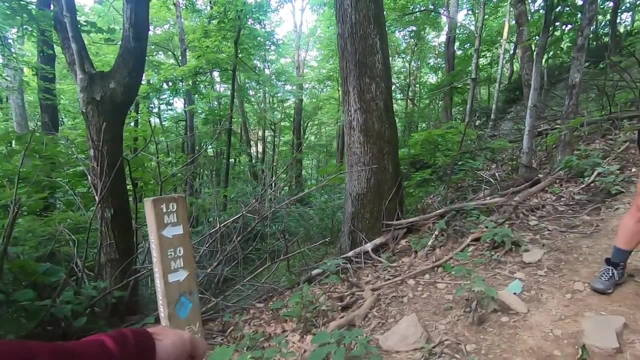 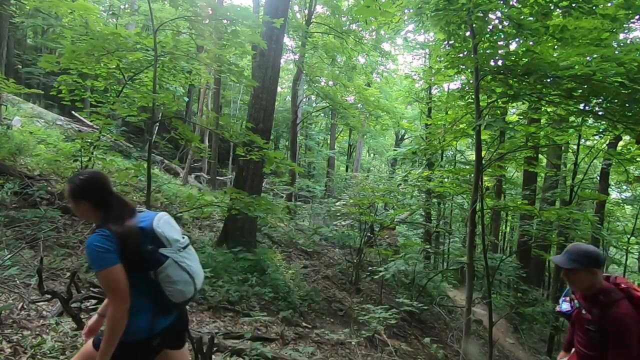 So another half mile, but we did 350 foot elevation gain instead of the initial 200.. We're getting there, It's being done on time. We're going to ride 100 miles and we're almost there. We're riding to the next point, but we don't see the Black Mountain. 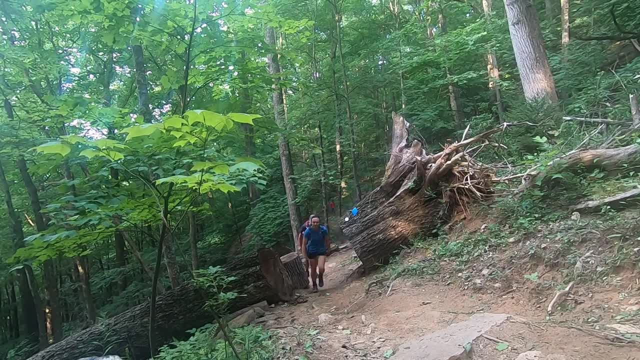 We'll run out and we will get back on track. Come on, Come on. This is fun. This is our first time. Yeah, This is the last trek we've done in the first month, but we've done some pretty good. 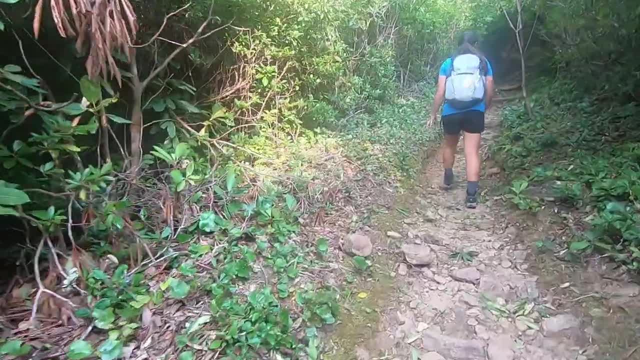 So we've got a nice set of wheels And the last thing we've done is we've gone up a good amount, We've gone up a good limit. It's already climbing up the hill. Yeah, We've done 1,300 feet. 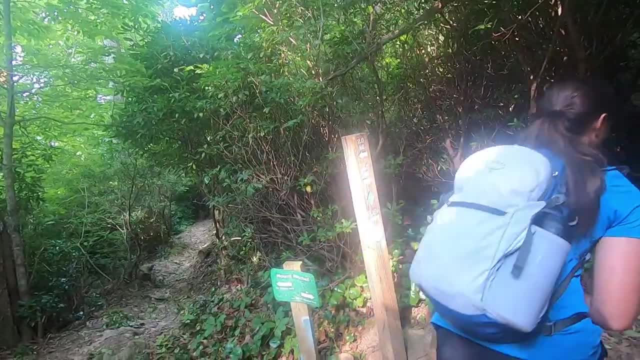 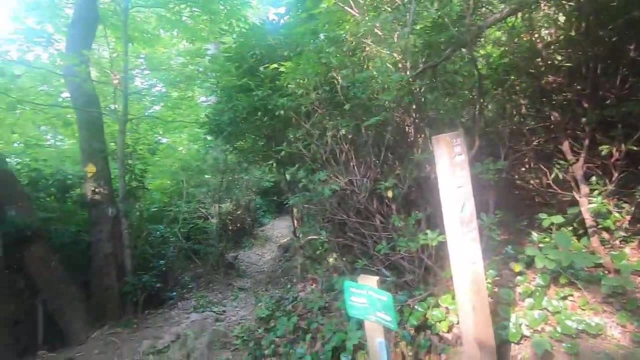 But it's hard to get on a mountain like this, But the falling down this hill is pretty good. Yeah, it is. The Prozent Hill Trail was amazing: 1,300 feet. We've done two miles. This is great, these little markers. 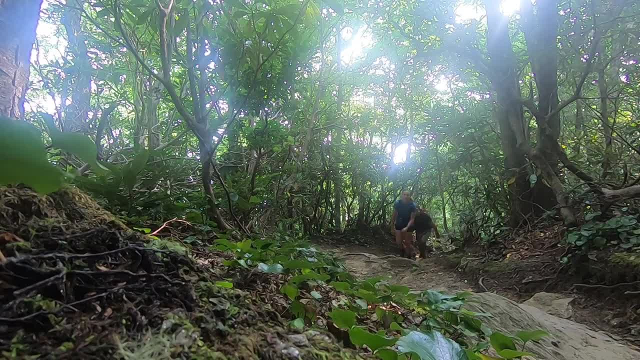 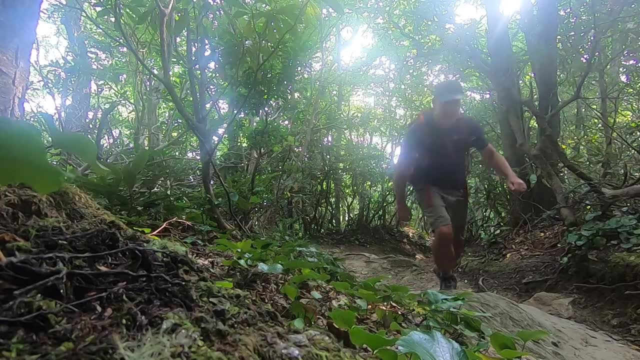 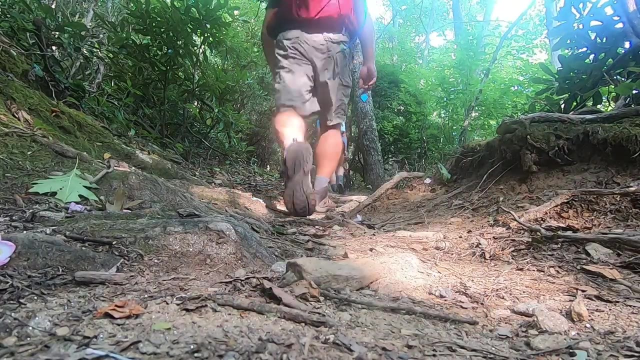 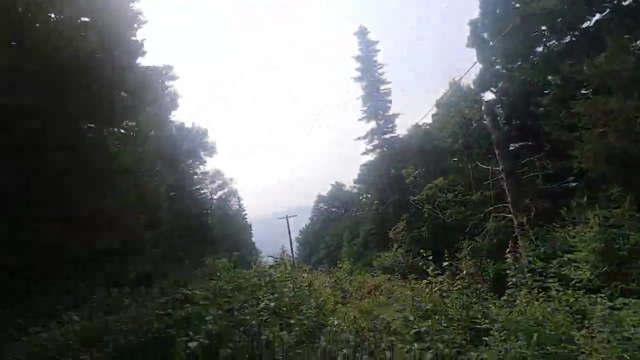 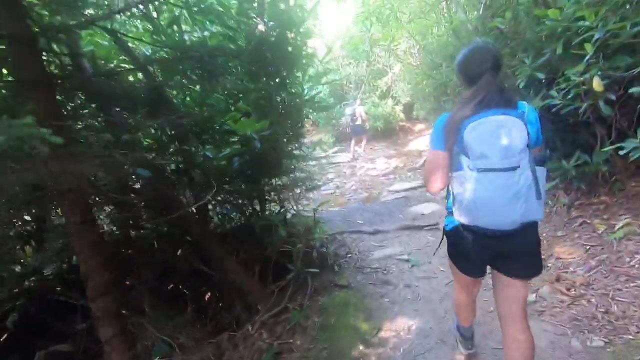 It is, and it's very well cleared. That opens up a little bit because of the power lines. Oh, some water, See, it does probably get fished. That's good and chilly, Is it? Yeah, it's good. 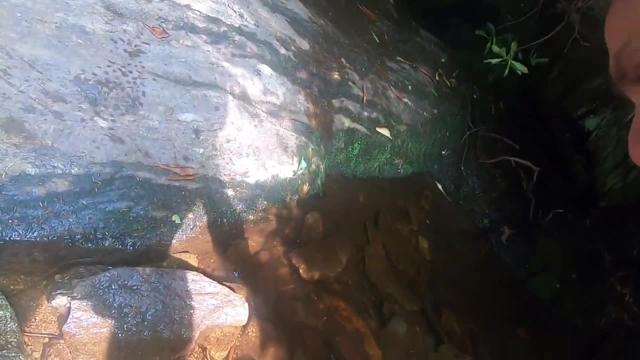 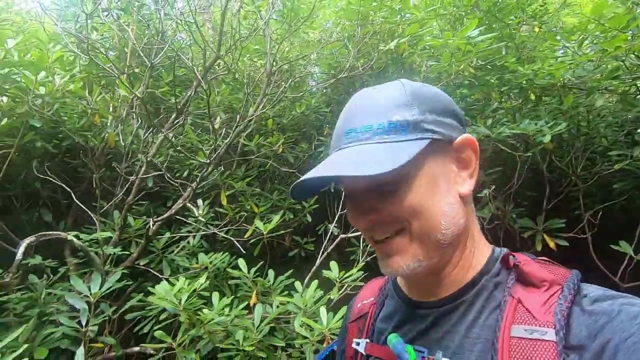 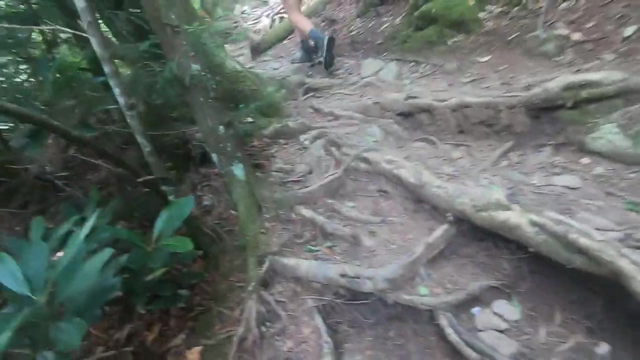 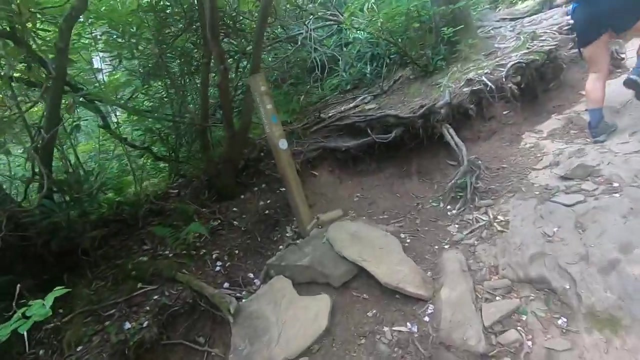 Oh wow, I think this is a rat eye. good, Oh wow. Because of this ascent and this distance, I think it is popular for those who are looking for exercise. Oh, we're at three. All right, we just passed the halfway point. 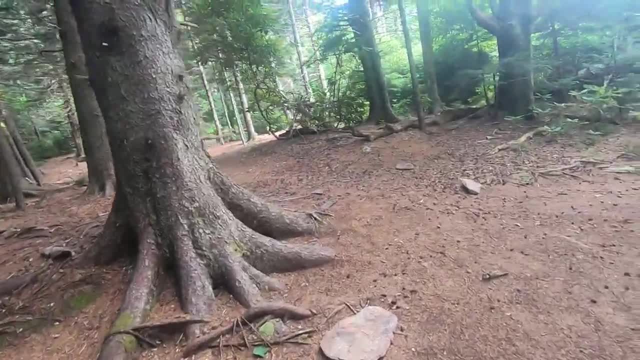 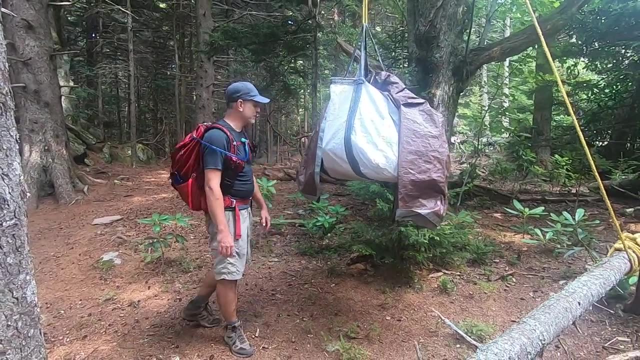 Passed by a few sites, I think, where you can do some camping- flat enough open areas We noticed near the campsites around here. we got some nice bags here That you can put your food in, things that you need to keep away from the bears. 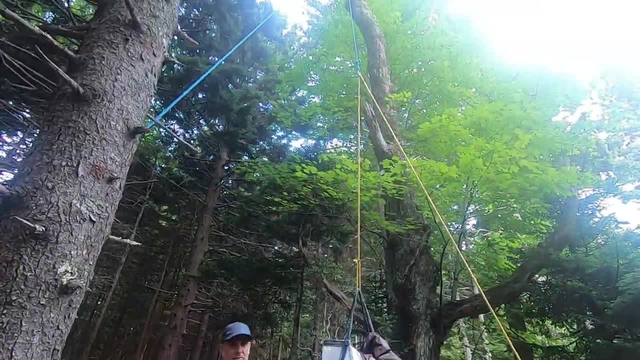 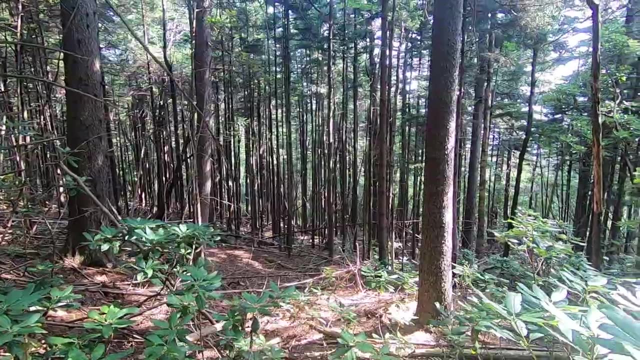 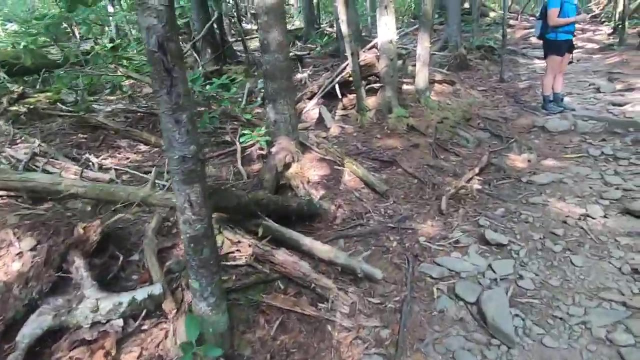 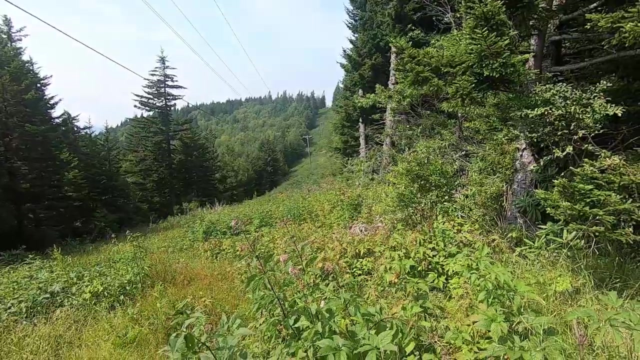 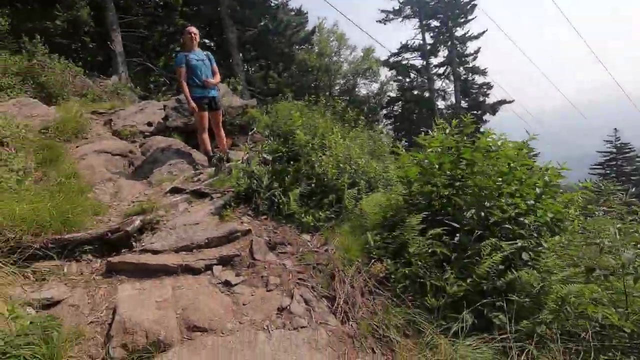 The ropes and stuff help you Pull the up there and you can just pull it up and get it well away from the bear's reach. Another milestone: It's a bunny. I did not expect that to happen. That's my feeling. I hope the best is yet to come. 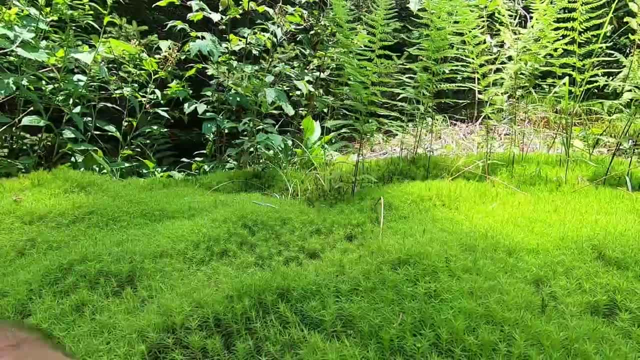 There, we're there. That's the good stuff. I'm going to go up there and try and do this jump. Oh, is that a bunny? Yeah, But this is a little too different. But I'll do it Okay. 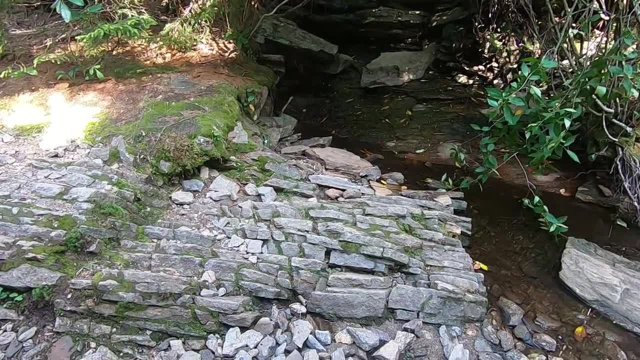 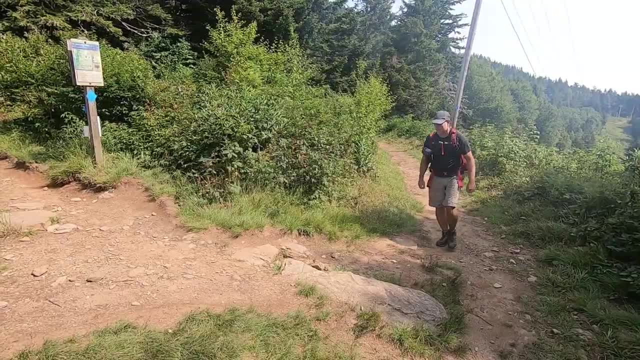 So it's not going to be that see-through. It's a little too rough. We're done All right. All right, All right, Let's do this. Wow, it's going to be fun, It's going to be funny. 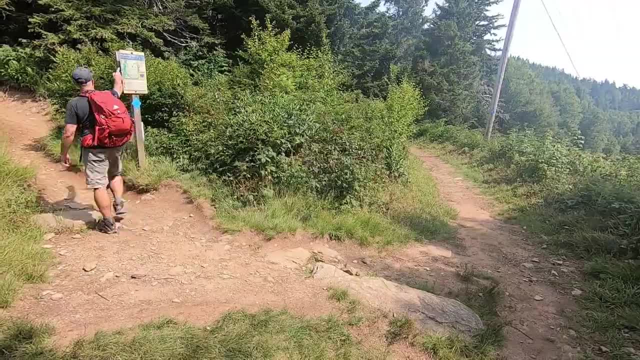 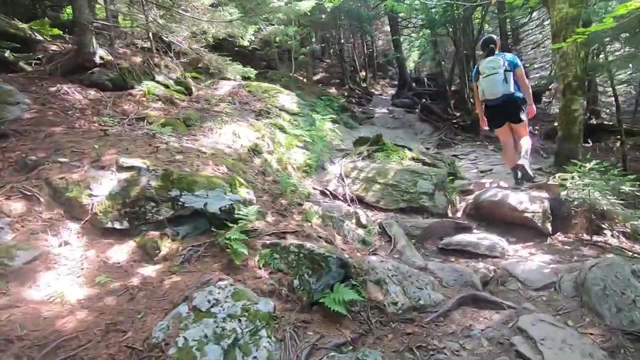 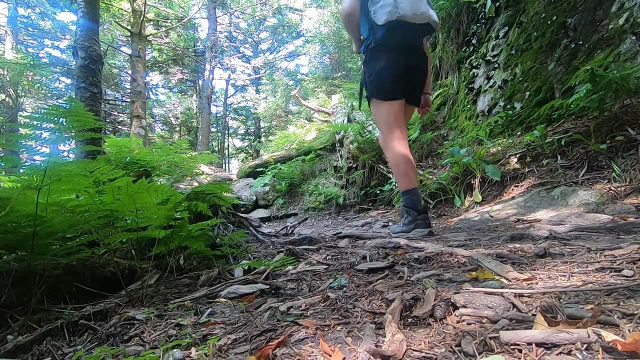 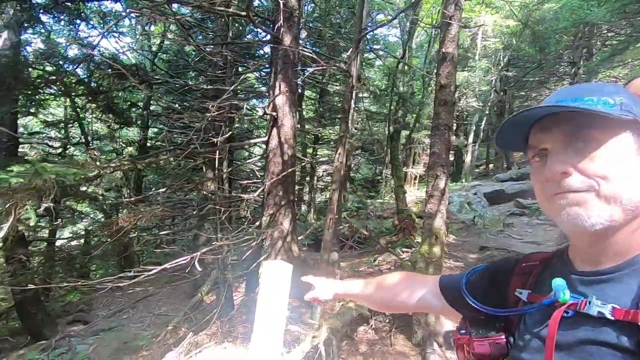 I'm going to do this. It's a little scary. Yeah, It's going to be fun. It's going to be funny. It's going to be funny. We're almost at 6,000 feet, Five mile mark. only one mile to go. 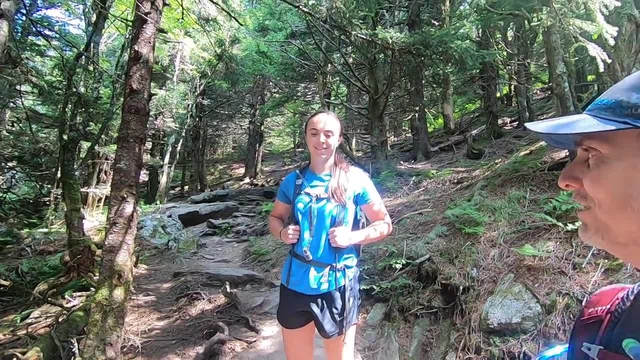 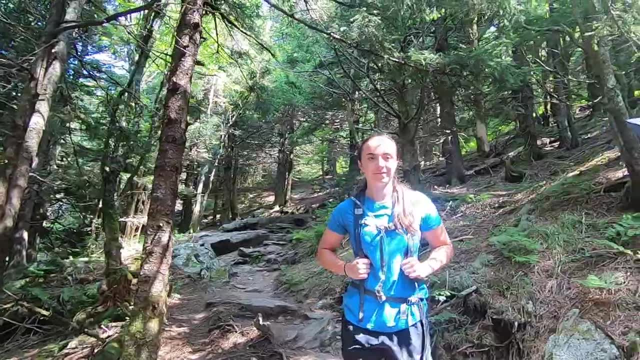 What's your impression of this hike, this trail? Not a lot of flat parts, Hardly any. A lot of loose rocks. We got a runner coming up. I think this is popular. That's one of the things that I've noticed. 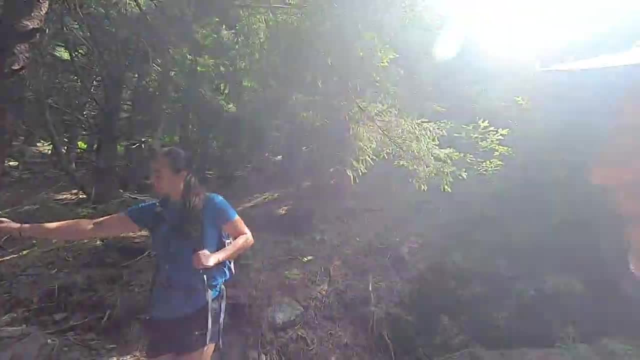 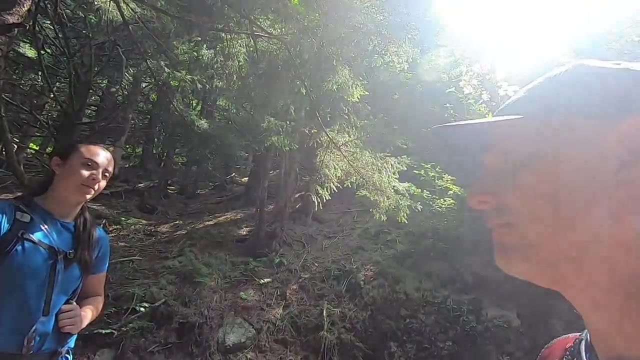 People to have six miles straight up. there's not a whole lot of places you could do that, So I think that's a popular thing to see. We're keeping a pretty good pace, but we're seeing more people passing us than we're passing. 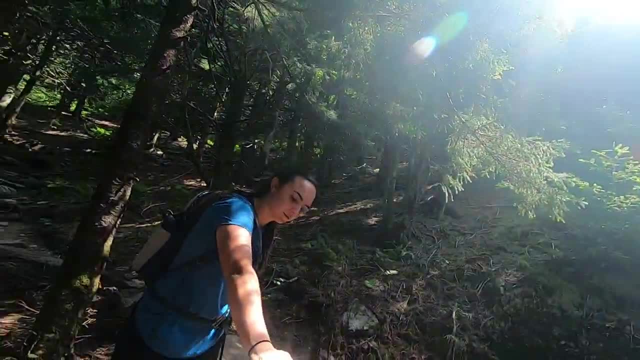 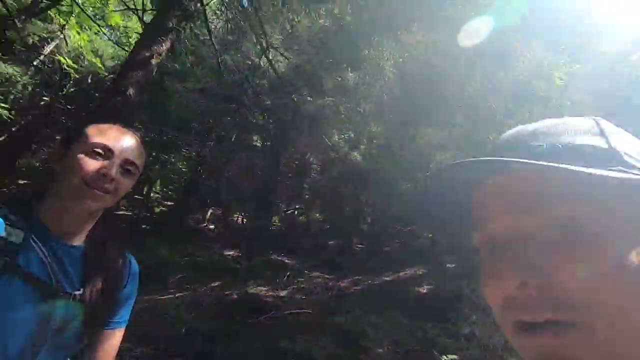 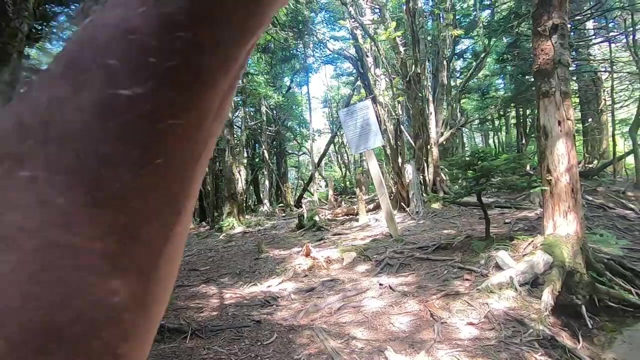 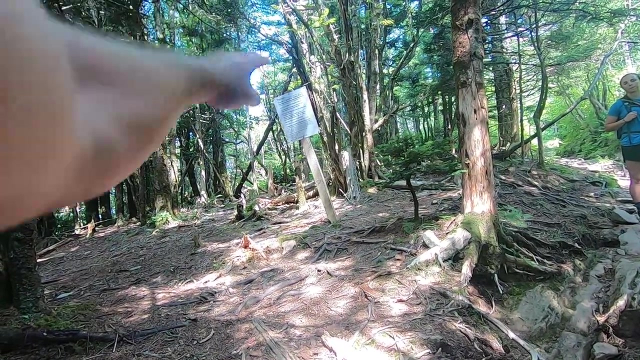 them. So it's not a trail that people take lightly. The experienced folks- Yes, This is a trail for experienced folks and we definitely notice that for the ones that are on the trail, I think here past the five mile mark, so we're within a mile of the peak. we're actually 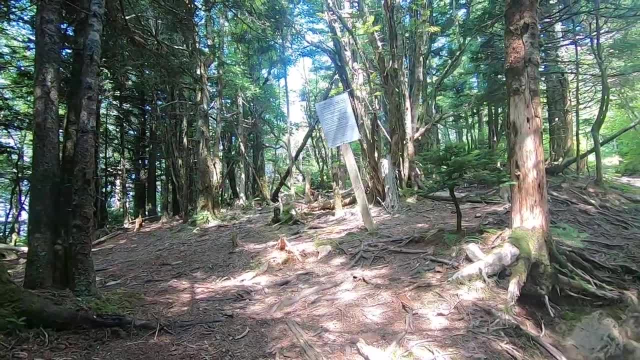 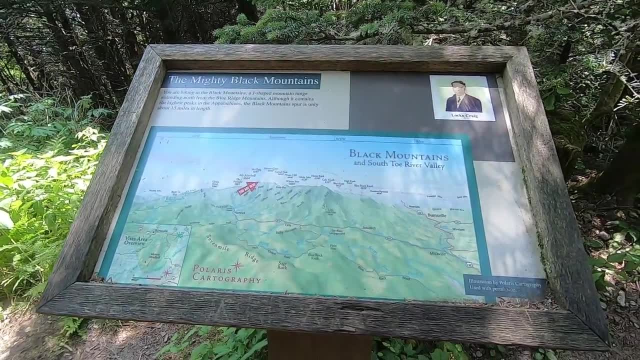 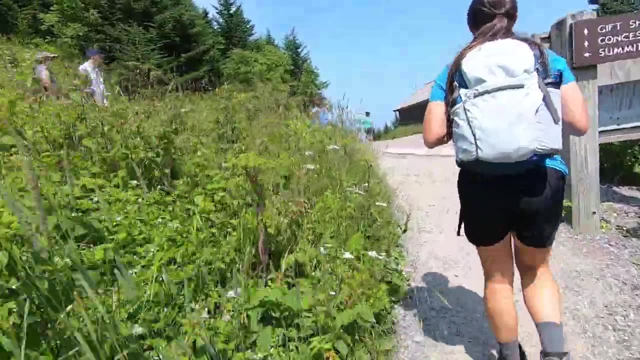 entering the trail, The Mount Mitchell State Park, Mighty Black Mountains, All right, Yeah, I wasn't exactly sure where we'd come out of. Oh, I see where we're at The summit's up here, so we're almost there. 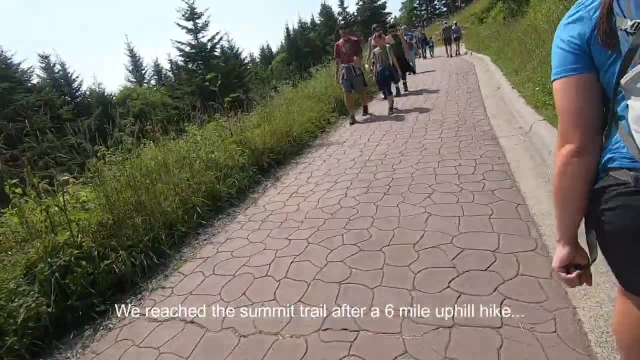 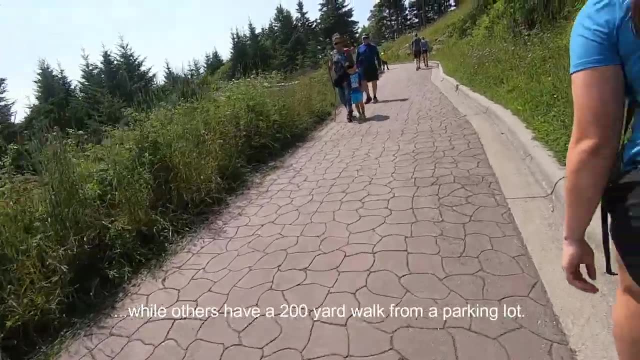 Yeah, this is. Oh, I see where we're at The summit's up here, So we're almost there. Yeah, This is: Yeah, We're almost there. Yeah, We're almost there. Yeah, Yeah, We're almost there. 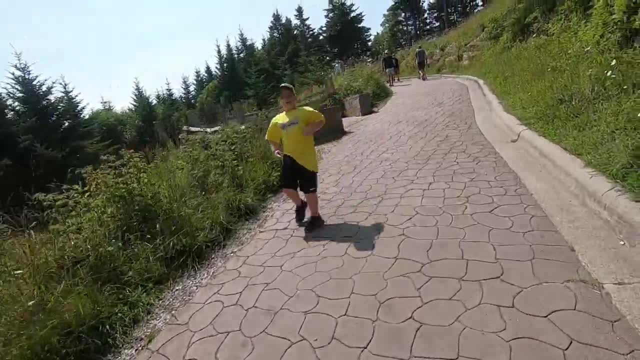 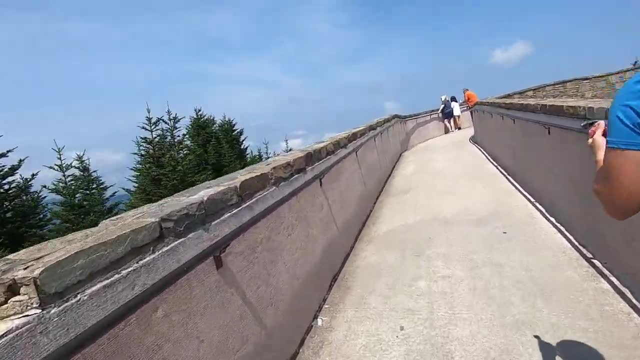 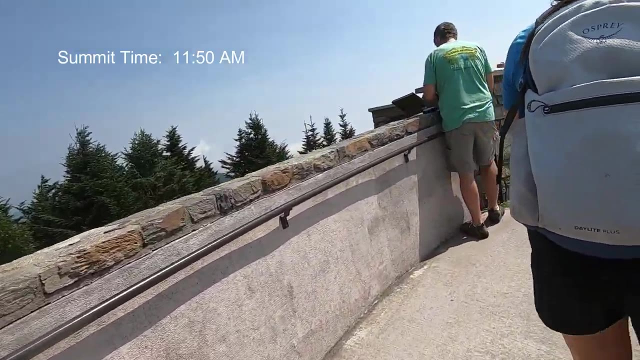 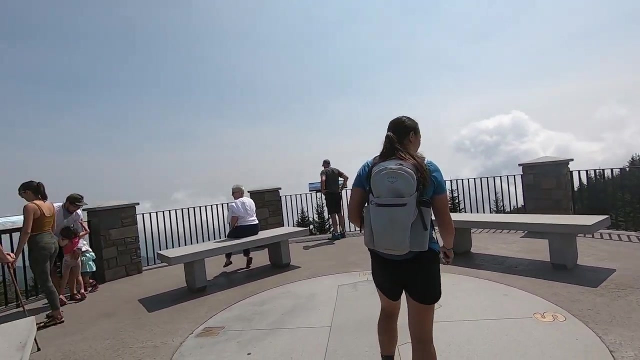 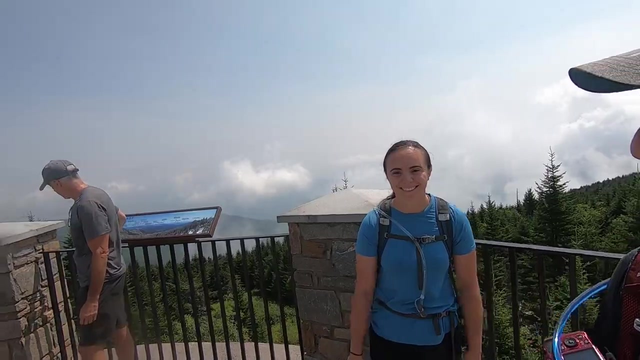 I think it's just funny. After hiking up six miles, We made it. We made it by 12.. 30 minutes ahead of schedule. 40 minutes, 40 minutes ahead of schedule. Yeah, We're crushing it. We crushed the gnarly hike. 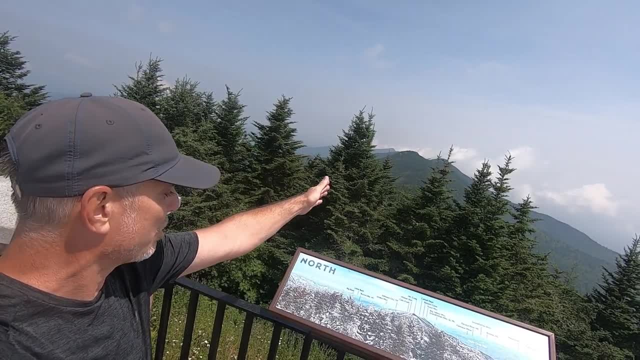 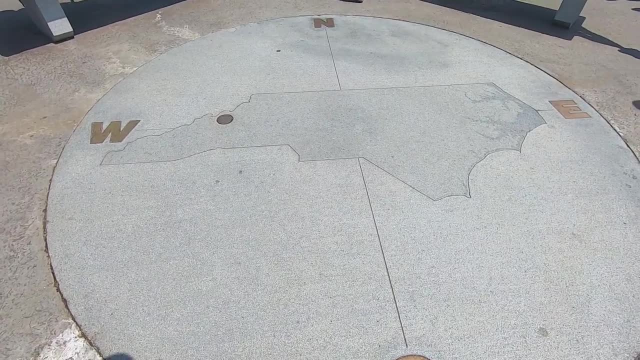 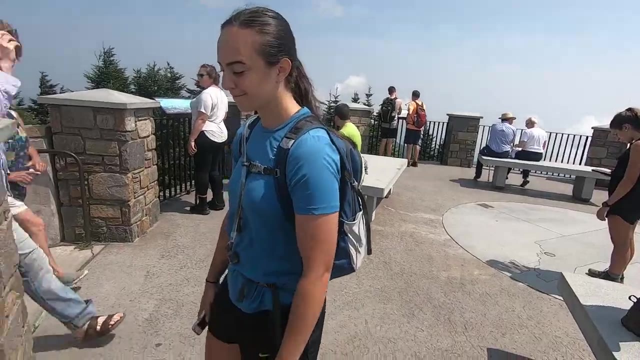 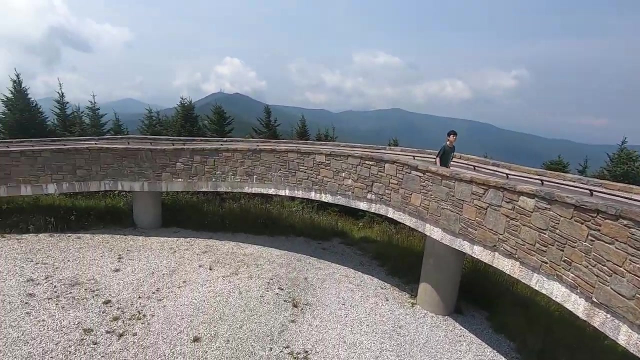 We got Mt Craig and balsam cones and the other peaks of the Black Mountains. So there's our state, right over there, The peak. This is it, this overlook area. you can kind of see how this curves around, goes down to the bottom. you got some signage down there. 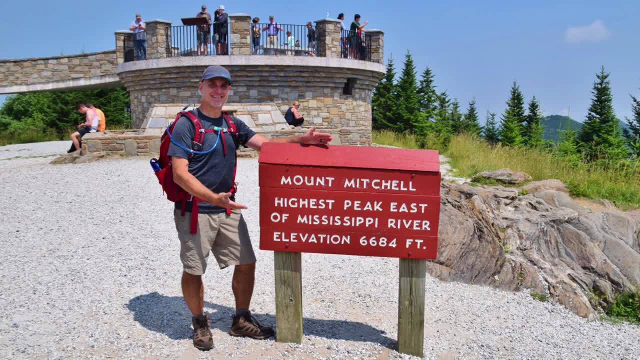 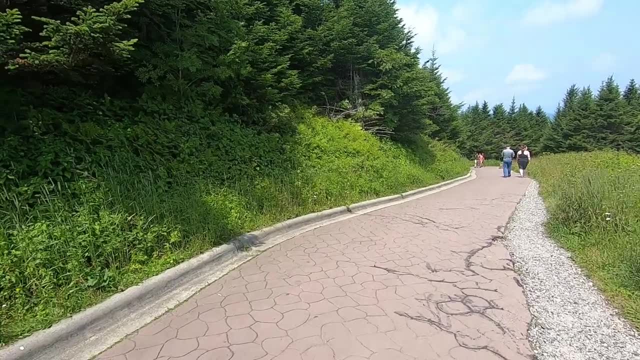 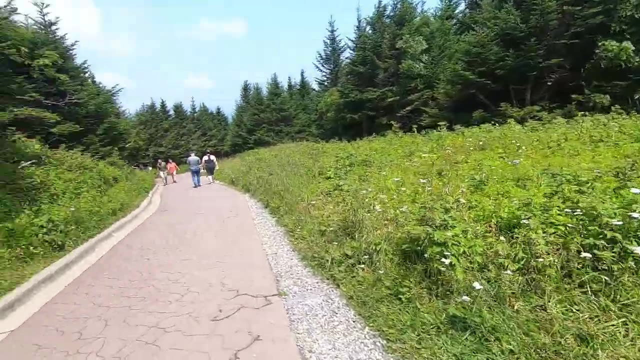 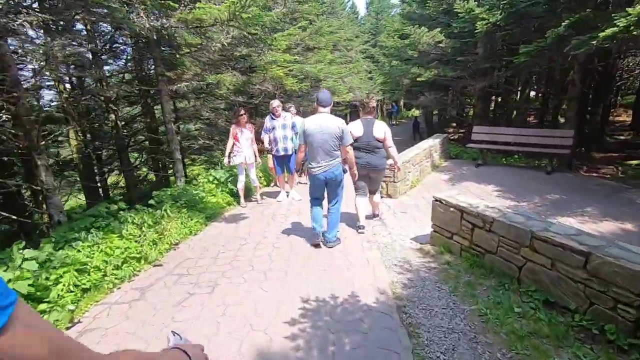 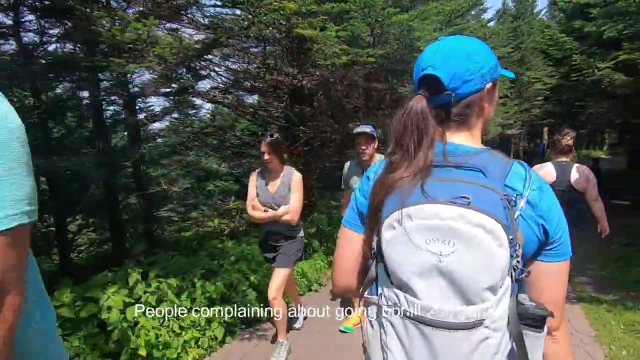 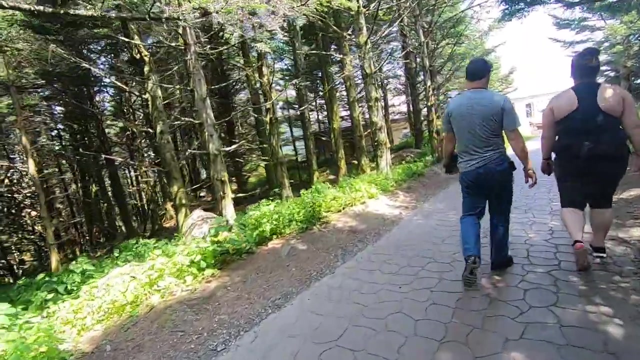 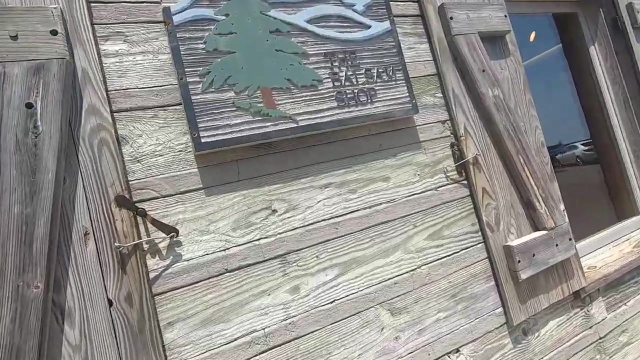 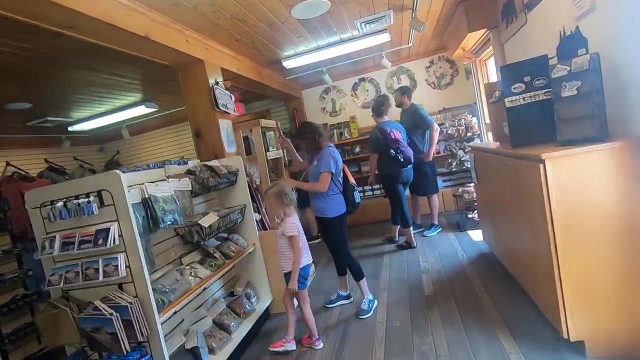 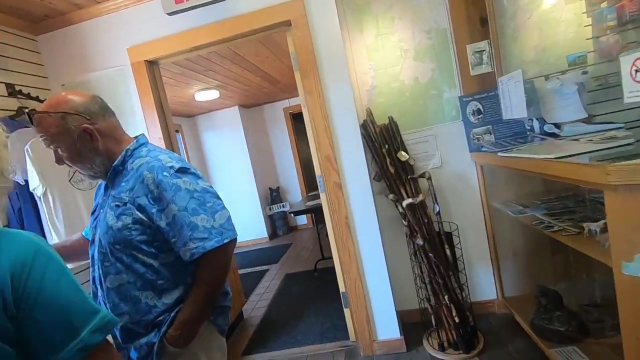 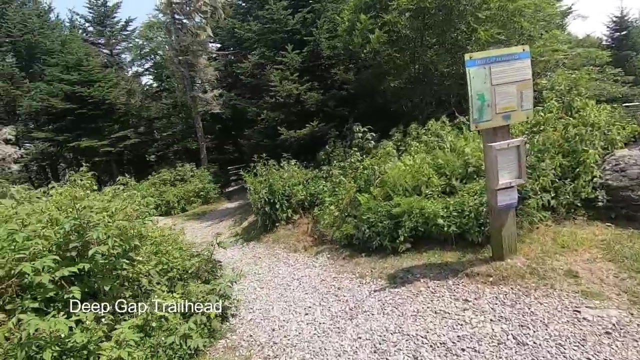 so now we're gonna go downhill here. i guess to go back we're gonna have to come back up here a couple hundred yards. good news is it's all downhill coming back. is that humorous to hear that someone complained about the 200 yard stretch. yeah, right here. 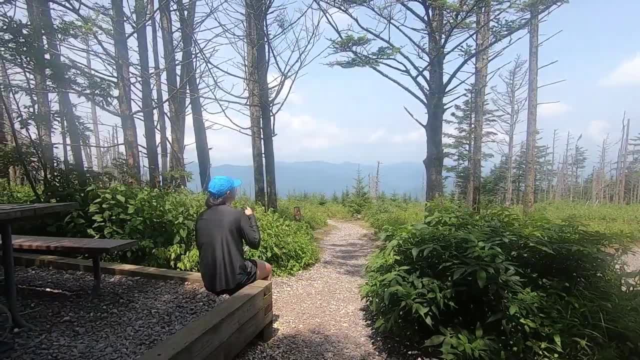 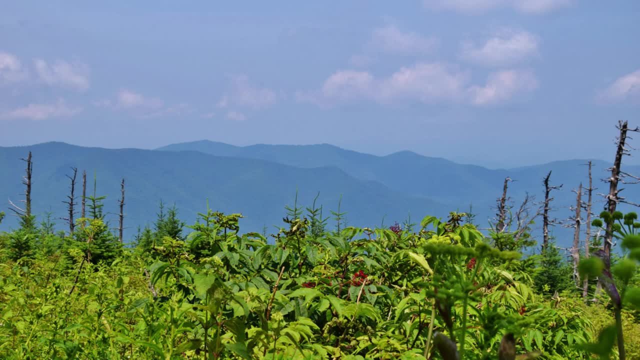 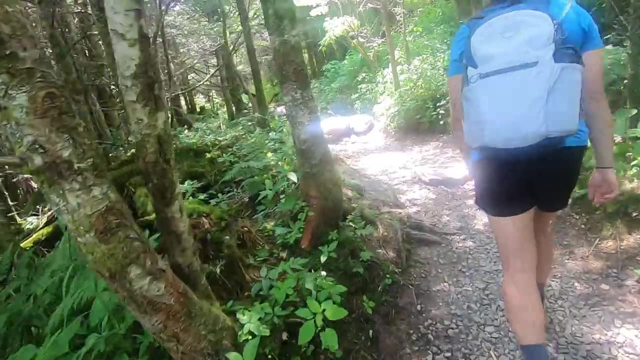 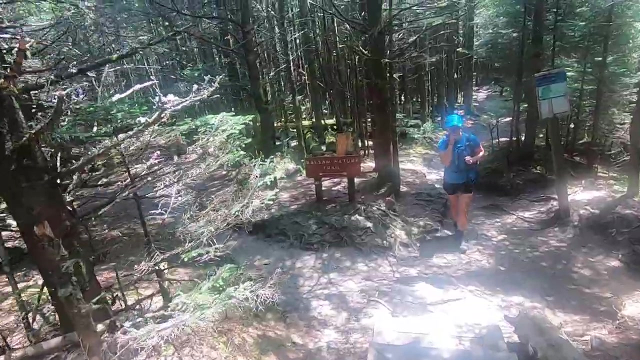 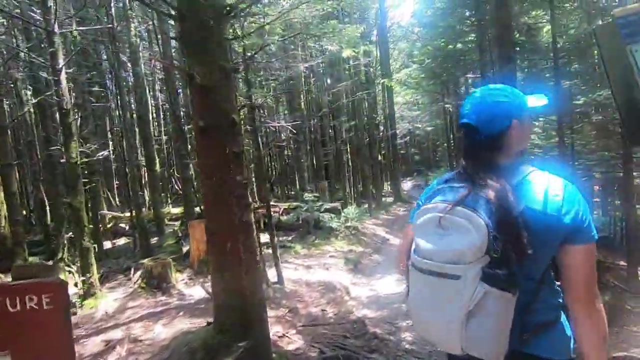 it's okay. we are headed back down six miles downhill. i'm not sure if i'm gonna like this any better. so we got the balsam nature trail that heads off in that direction, but we're gonna stay on mount mitchell trail. sun kind of opens up right there. 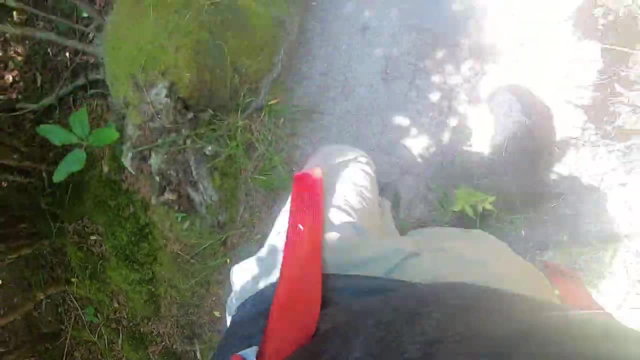 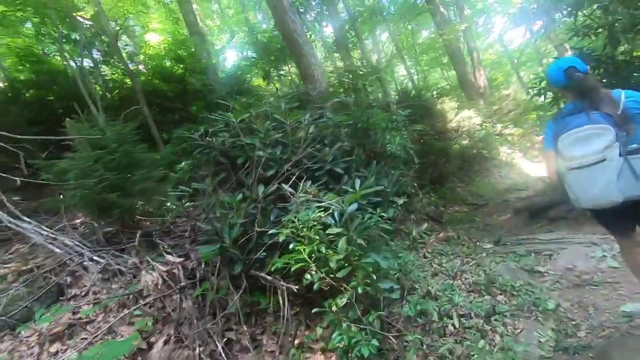 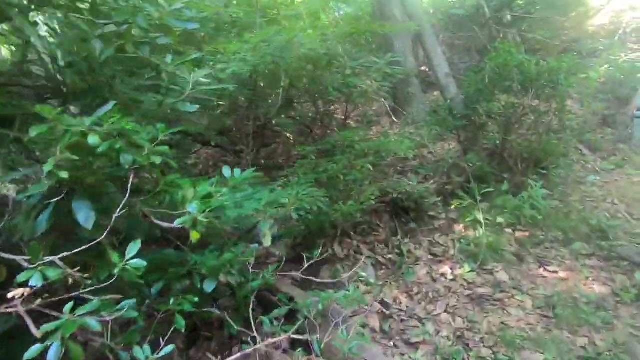 what will take after two days. i was working hard going up but my legs never felt like jello, i mean they never felt wobbly going up. it was uh, you know, i had to stop, maybe catch my breath or something, get a drink of water, but here 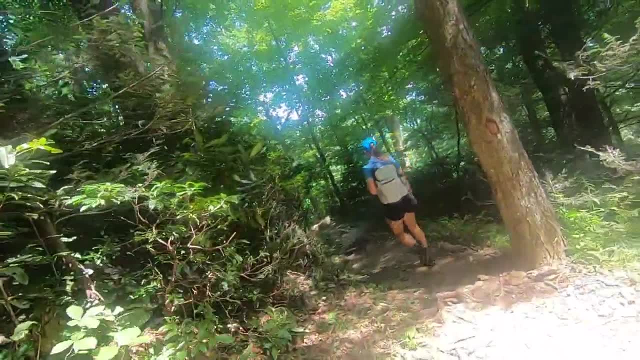 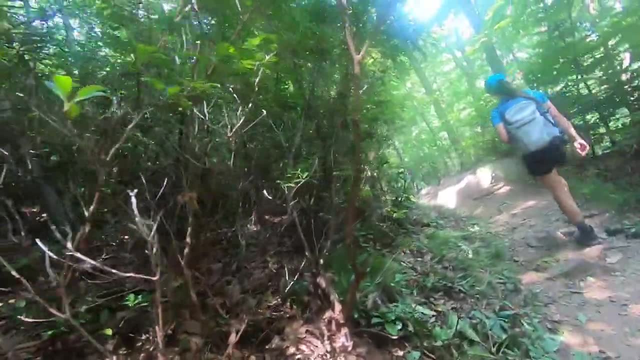 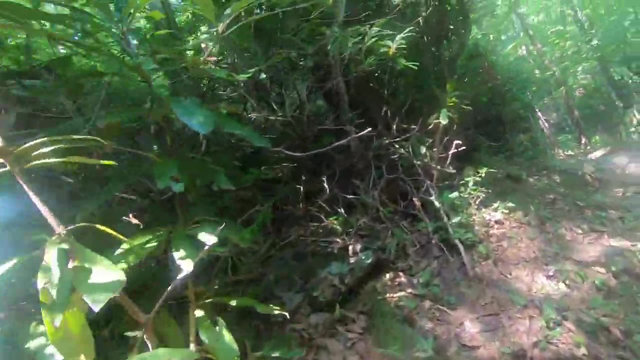 it's like: yeah, my legs are wobbly bigger. yeah, yeah, estimate the downhill portion of this hike. it's still has its own challenges, especially if you have any knee issues or anything like that. so, but and your toe is getting crammed up in the front of your shoes, which is why I did not.